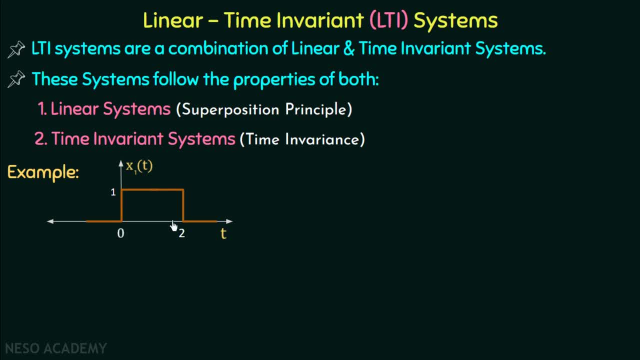 x1, t is a function which is having a rectangular waveform from zero to two And it is given as an input to the LTI system And its response is y1, t, x2, t is another function which is having this waveform And it is given to the same LTI system And it gives the same LTI system And it gives the. 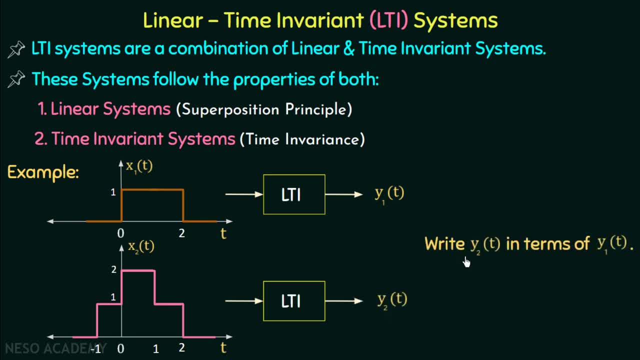 the response y2t. Now we need to write y2t in terms of y1t, where y2t is the response of LTI system when x2t is given as an input and y1t is the response of same LTI system when x1t is given. 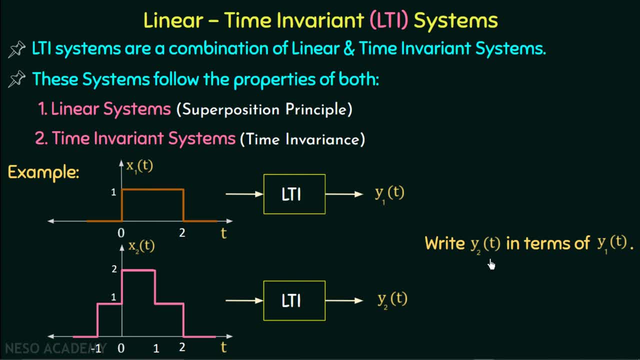 as an input. So they are asking the relationship between y2t and y1t. In that case there must be a relationship between x2t and x1t. So now I want you all to pause this video and try to figure. 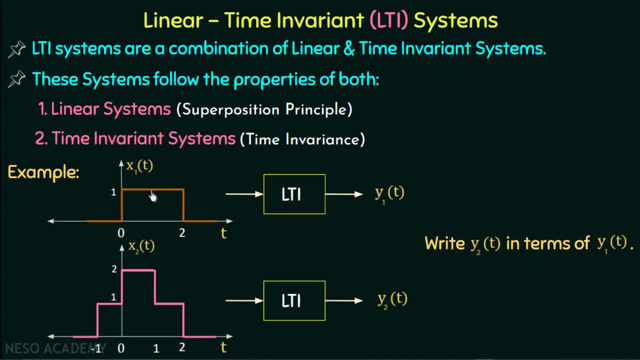 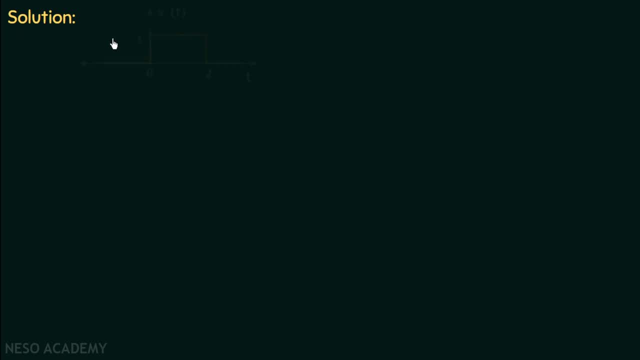 out the relationship between x2t and x1t And then, after that, we will move on to the solution. Now, moving on to the solution we are given, x1t, which is having a rectangular waveform from 0 to 2,. 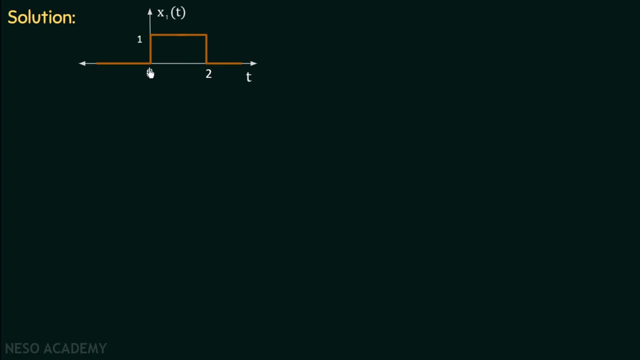 that is, the value of this function from minus infinity to 0 is equal to 0, the value from 0 to 2 is equal to 1.. And the value from 2 to infinity is 0.. Now, if I time shift this function on the left-hand side. 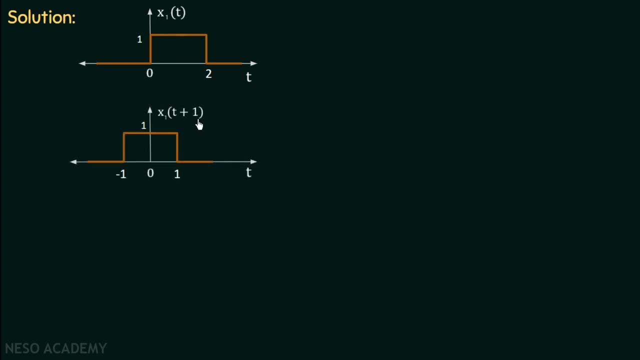 by a factor of 1, then we will get x1 of t plus 1 and its waveform will be a rectangular function from minus 1 to 1.. If I time shift this function on the left-hand side by a factor of 1,, then 0. 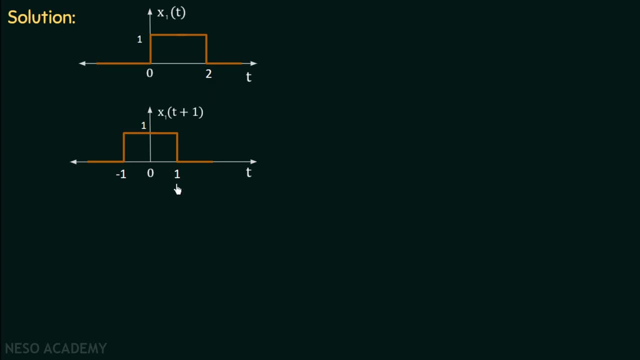 will shift to minus 1 and 2 will shift to 1.. And that's why its value from minus infinity to minus 1 will be equal to 0.. The value from minus 1 to 1 will be equal to 1 and the value from 1 to infinity will be equal. 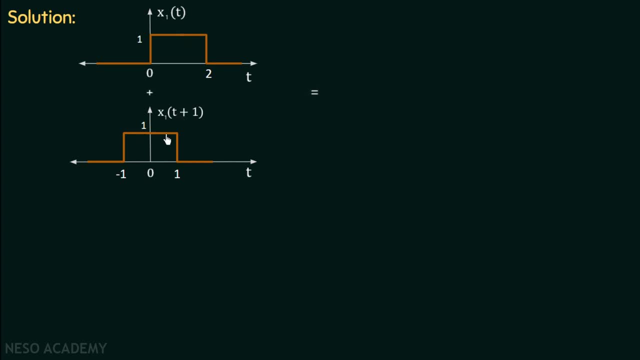 to 0.. So now we are going to add these two functions and let's see what is the resultant waveform. So the value of x1t plus 1, from minus infinity to minus 1, is equal to 0, and the value 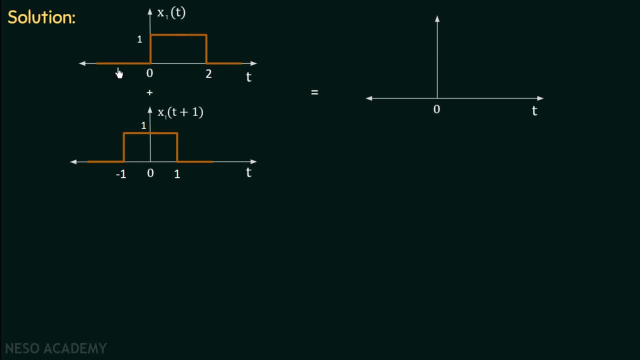 of this function from minus infinity to minus 1 is equal to 0. So if we add these two functions from minus infinity to minus 1, we will get the resultant value equal to 0.. So if we add these two functions from minus infinity to minus infinity, 0, the value of x1t plus 1 before including. 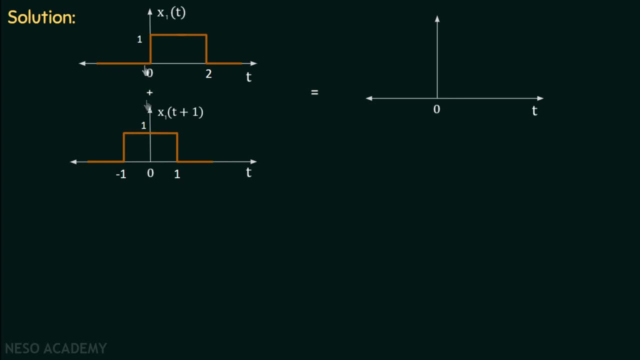 there, x1t plus 1. from minus infinity to minus infinity, 6 is equal to 0. And from minus 1 to 0,, this function is equal to 1, and this function is equal to 0.. So if we add these, 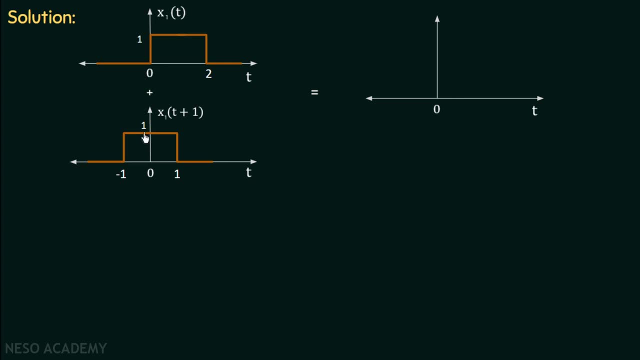 two functions, then 1 plus 0 will be equal to 1.. So the resultant waveform in the left-hand side will look like this: It will be equal to 0 from minus infinity to minus 1, and it will be equal to 1 from minus 1 to 0. Now 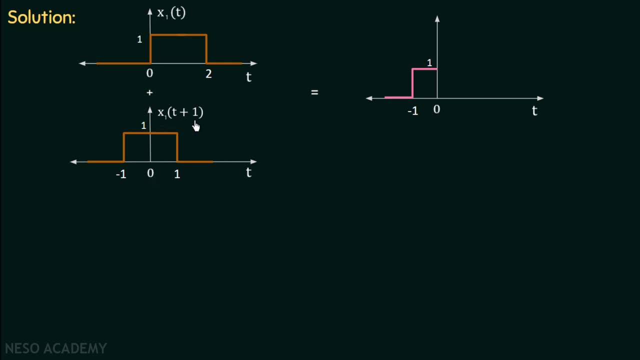 moving on to the interval from 0 to 1, x1t plus 1 is having the value equal to 1 and also having the value equal to 1 because it is having the value equal to 1 from 0 to 2.. 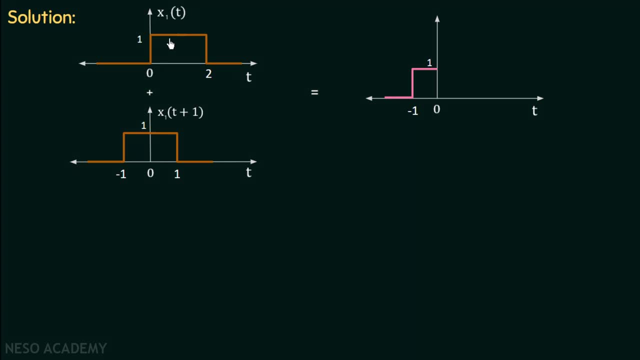 So if we add these two functions from 0 to 1, 1 plus 1 will be equal to 2.. So the resultant value from 0 to 1 will be equal to 2.. Now, moving on to the next interval, from 1 to 2,. x1 is having: 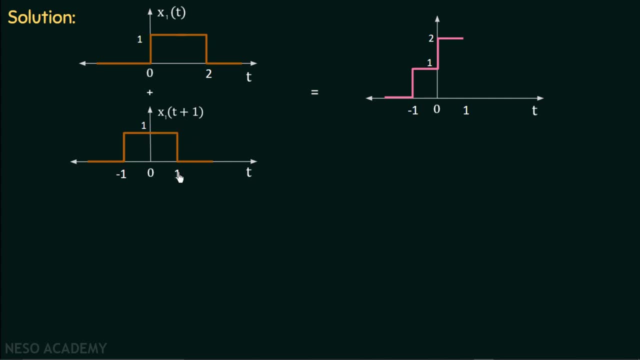 the value equal to 1 and x1 is having the value equal to 0. So if we add these two functions, then the resultant value from 1 to 2 will be equal to 1.. And now, from 2 to infinity, the value. 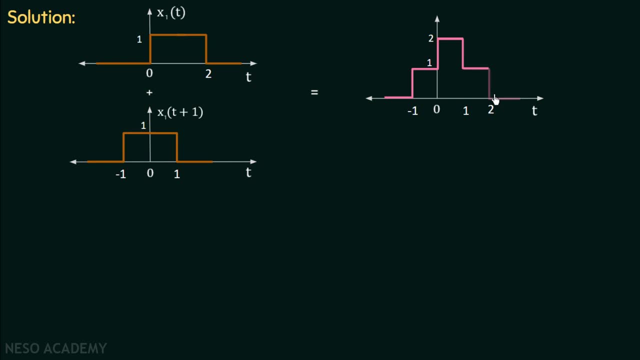 of both the functions are equal to 0. That's why the resultant value will also be equal to 0.. And now we have got our final waveform after adding these two functions, And if we observe this waveform, this is the waveform of x2. So we can say that x2 is the sum of x1 and x1 plus 1.. 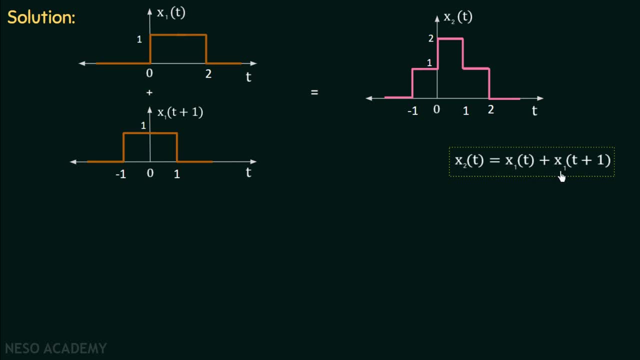 So x2 is equal to x1 plus x1. So we can say that x2 waveform is the linear combination of x1 and x1. Now if we are having an LTI system and if I give x1 as the input to the LTI system, then the response is equal to y1 according to the example. Now if I give: 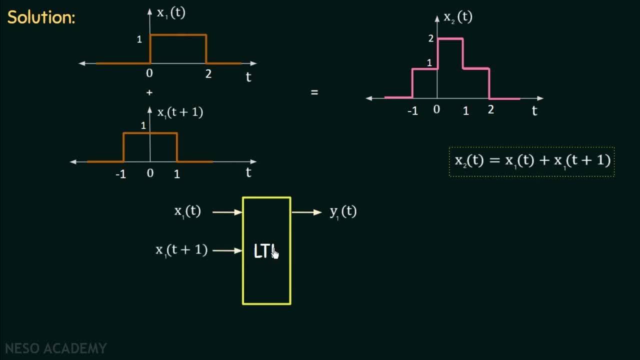 x1 as the input to the same LTI system, then by time invariance property, the response will be equal to y1, which is the time-shifted version of the response of x1. Now if I add these two functions, then we will have x1 plus x1 and. 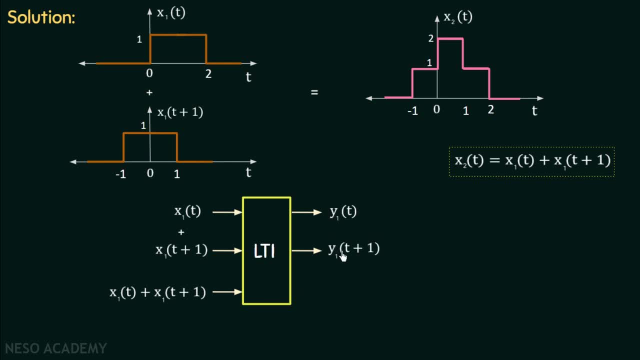 by linearity property. its response will be the individual addition of these two responses and it will be equal to y1 plus y1. This is the property of an LTI system. It is following the properties of both the linear systems and both the linear systems and we have 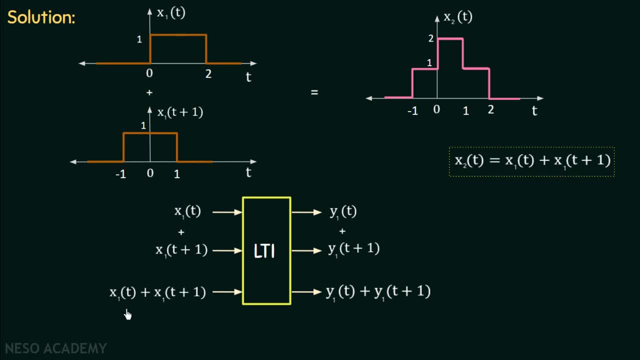 the time invariant systems. Now x1 t plus x1 t plus 1 is equal to x2 t. So we can say that y1 t plus y1 t plus 1 is equal to y2 t. In this way we have written y2 t in terms of y1 t. So now we 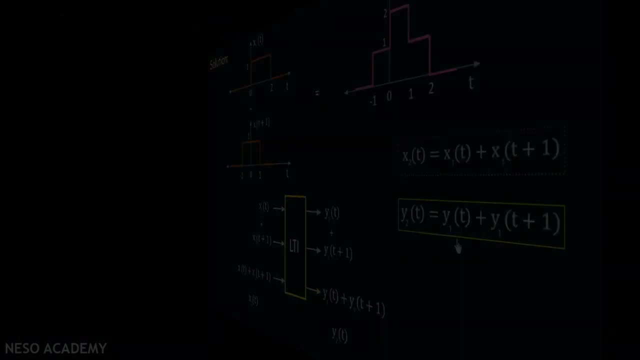 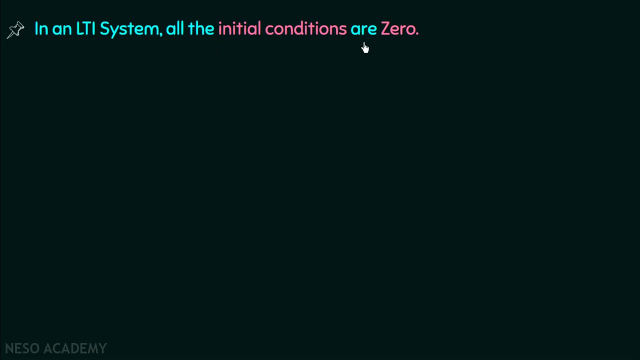 are done with this example, We will now move on to the next point. The next point of our discussion is given: as in an LTI system, all the initial conditions are 0.. Now, this is one of the most important properties in LTI system: all the initial conditions must be equal to 0.. I'll 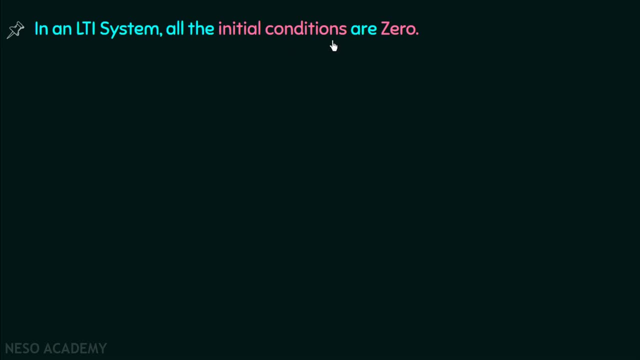 explain you what are the initial conditions. But firstly, we will understand the reason that why the initial conditions must be equal to 0 in the case of LTI systems. So the total output in any system is equal to ZIR plus ZSR. ZIR is the result of the initial conditions. So if we take this, 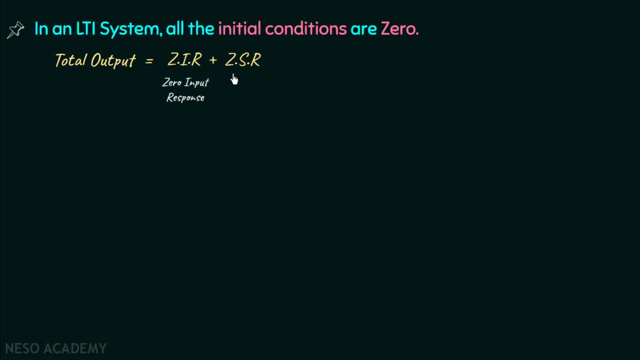 zero input response: the zero input response and ZSR is the zero state response. ZIR is the response of the system when the input is equal to zero and ZSR is the response of the system when the input is given to the system. So whenever we will give the input to the system, we will have the ZSR and 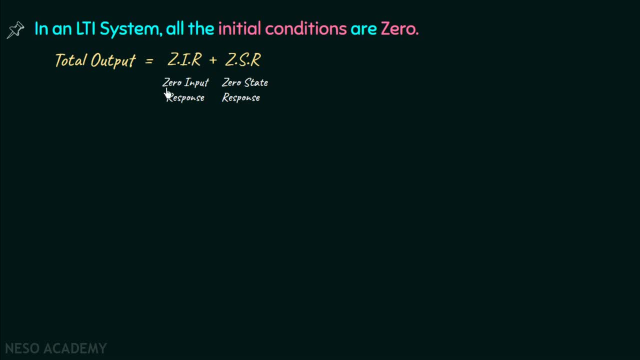 if the input is equal to zero, then the zero input response will come into the picture. The zero input response is due to the initial conditions of the system, And if the initial conditions are not zero, then the total output will not be equal to zero, it will be equal to ZIR. Now, in case of 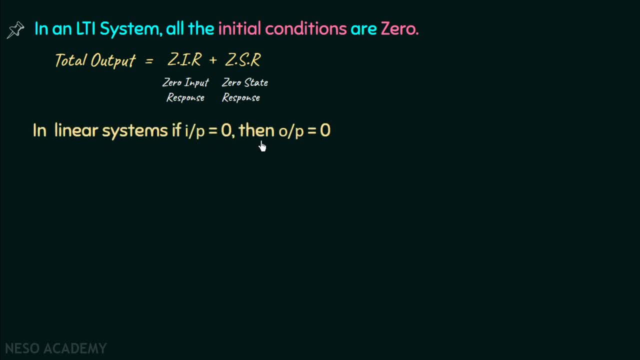 linear systems. if input is equal to zero, then output must be equal to zero. It is a property of linear systems that if input is equal to zero, then output must be equal to zero. That is, the initial conditions must be equal to zero, because if the 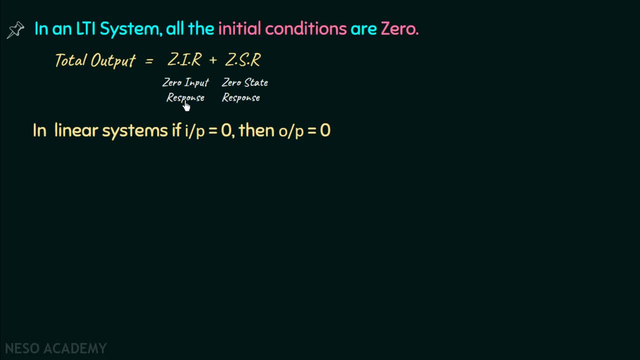 initial conditions are not equal to zero, then the zero input response will come into the picture. then the total output will not be equal to zero, it will be equal to ZIR. But in case of linear systems the output must be equal to zero. That is the total output in case of linear systems. 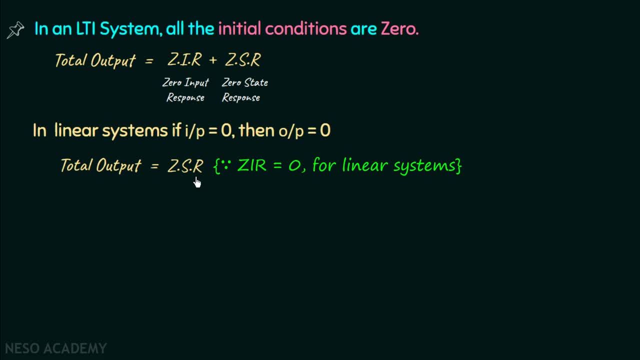 must be equal to ZSR. It means that whenever we will give the input to the linear systems, then only the output will come into the picture. Now suppose if the initial conditions are not zero, then in that case the zero input response will come into the picture. And if 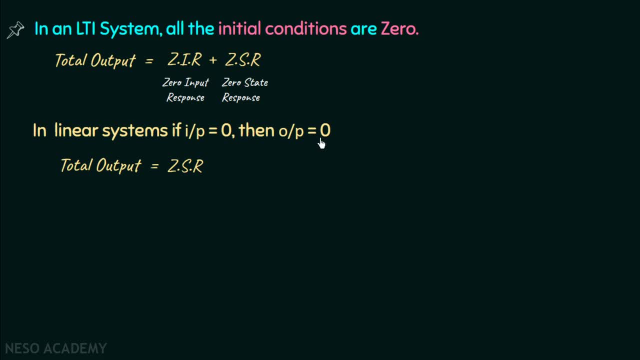 the input is equal to zero, then the output will not be equal to zero. And if the input equal to zero and output is not equal to zero, then the system will not be a linear system. And if the system is not linear, it will not be LTI. So we can say that for the system to be an LTI system, 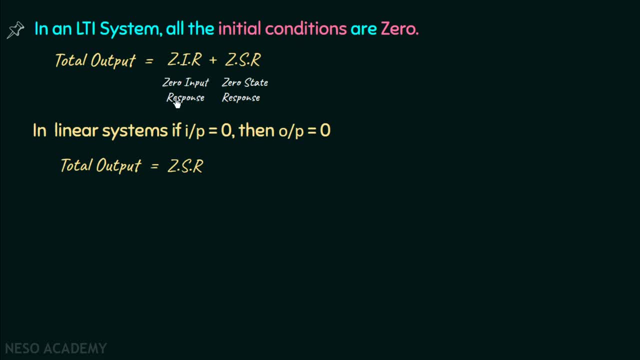 the initial conditions must be zero. the zero input response must not exist in the picture. So the zero input response must be equal to zero, That is the total output. and the total output must be equal to ZSR, That is the zero state response. This is the must condition. 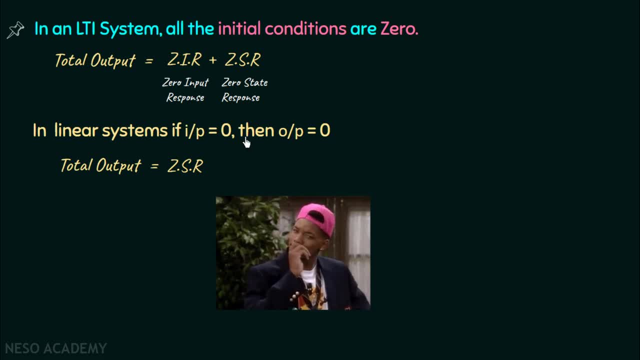 for an LTI system. Now you must be thinking that how we can get the output without applying the input, or what is the significance of this zero input response. So let's understand this with the help of this example. We all have torch lights in our homes and these torch lights run on. 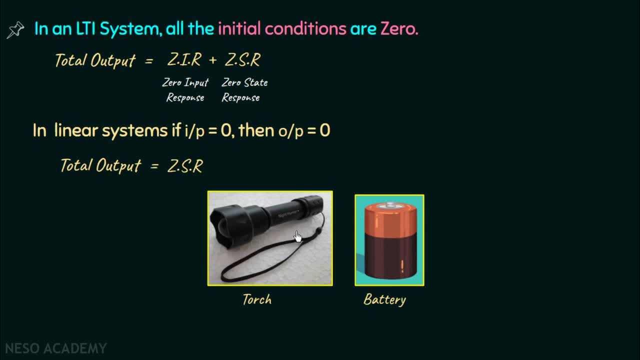 charges stored in them, which is the power source for this torch, and in this case we are not applying any external input to this system. so the charges present inside the capacitor of the battery are kind of an initial condition of this particular system and they are providing a zero. 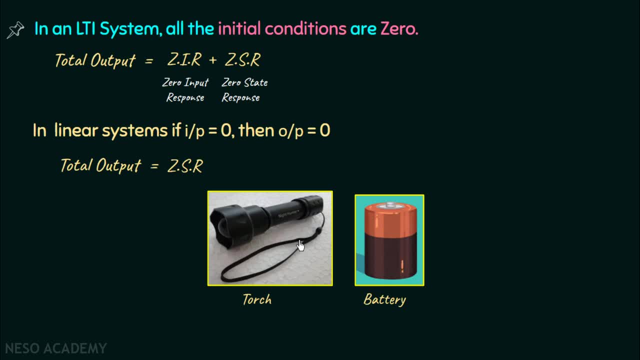 input response, because we are not providing any external input. the input is applied to the system when we need to charge this battery. so in this way we can have the output without applying an input due to the initial conditions of the system. so now i hope you have got the significance.